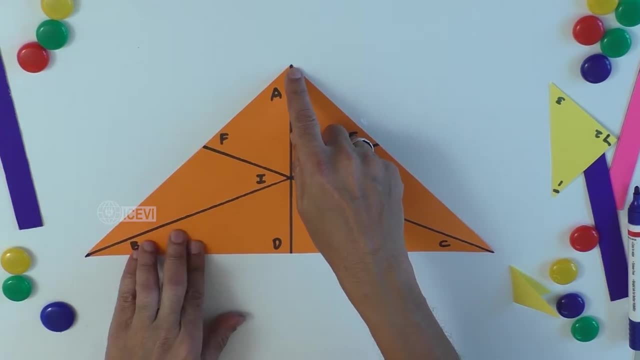 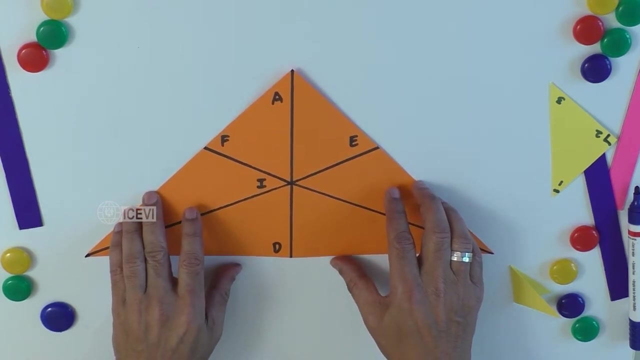 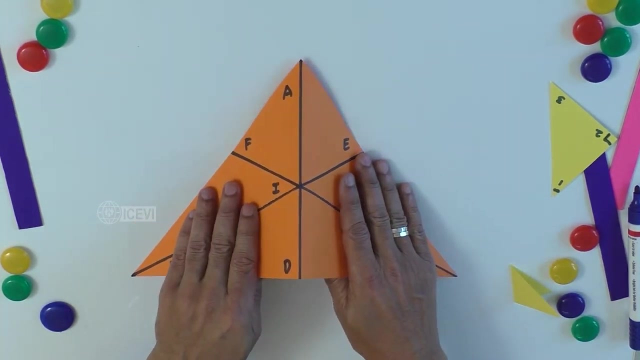 in-center. we have to find the angle bisector of A, angle bisector of B and angle bisector of C, and the meeting point becomes I. Now how to do that. instead of taking a measuring device and making each angle into two halves In paper folding technique, we have to simply fold the paper in such a way that the side AC is coinciding with the side AB. 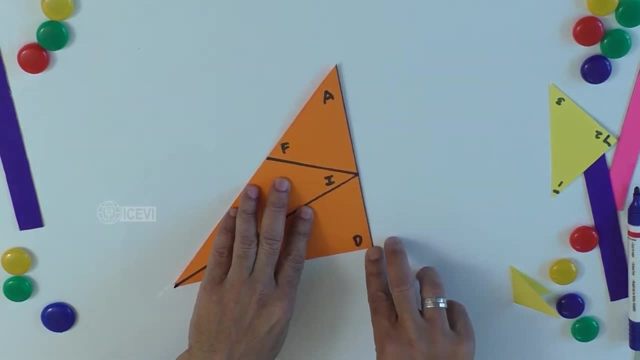 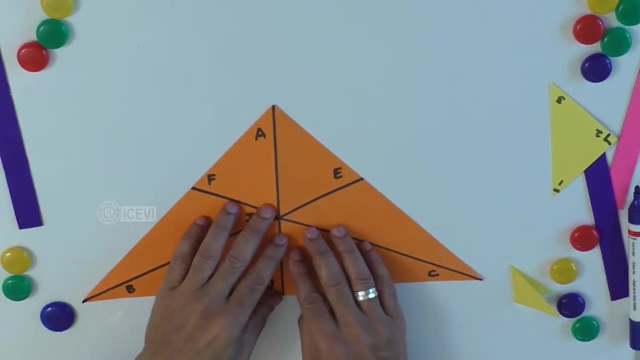 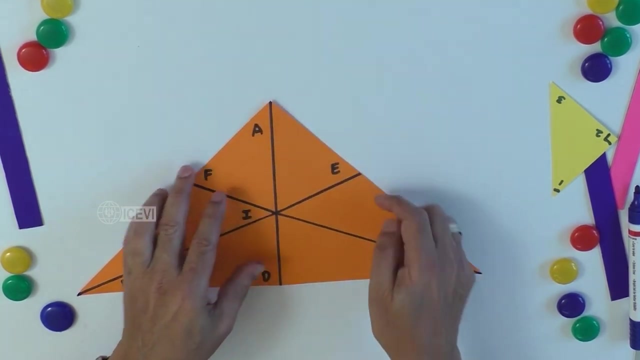 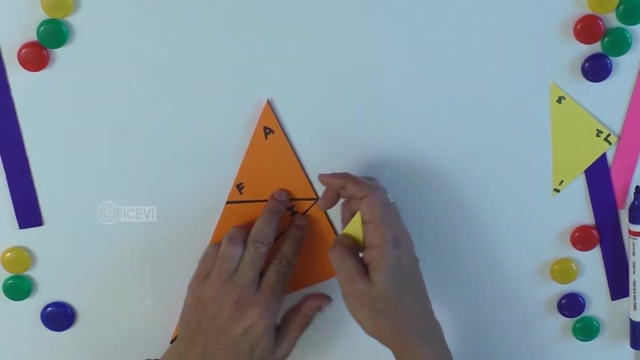 strong crease. fold the paper and make a strong crease. that will make the angle A into two halves. you can notice that this paper strip is angle A. when you fold the paper in such a way that AB is coinciding with AC, the angle A is. 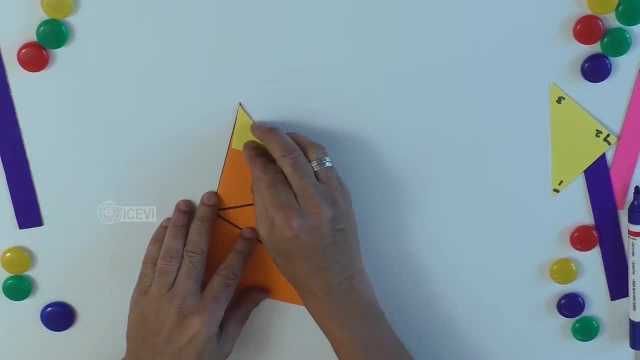 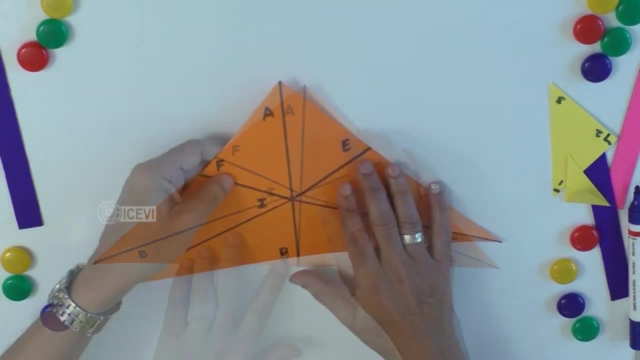 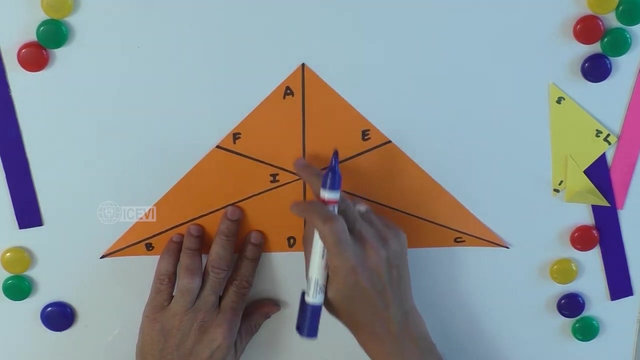 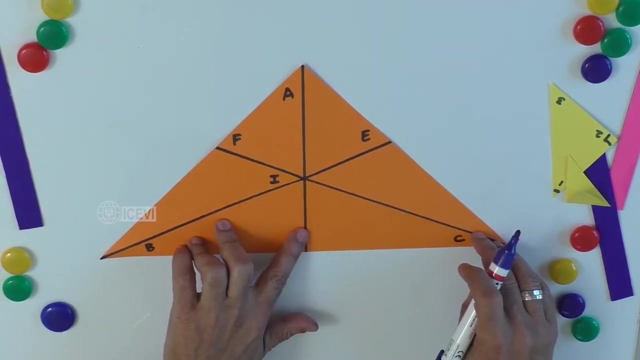 automatically made into two halves. similarly, you can measure angle bisectors C and B too. now you can notice that all the angle bisectors- AD is the angle bisector of angle A, BE is the angle bisector of angle B and CF is the angle bisector of angle C. they are going through a point which is: 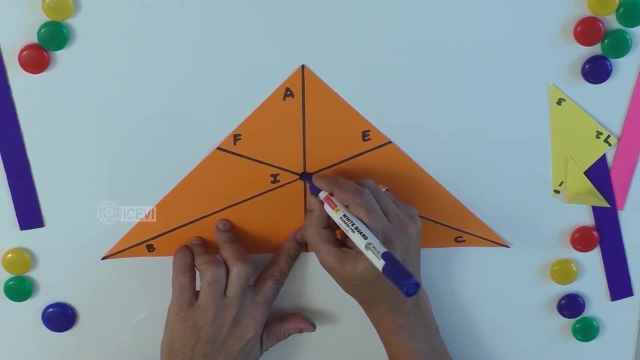 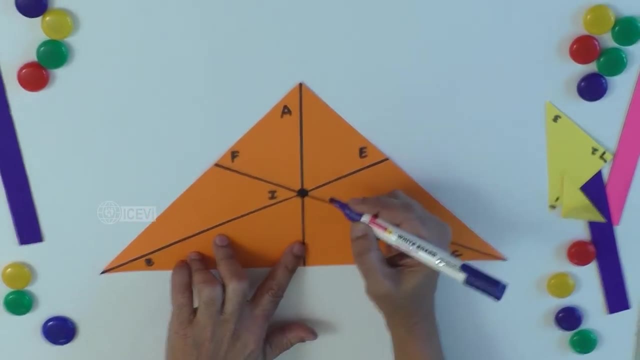 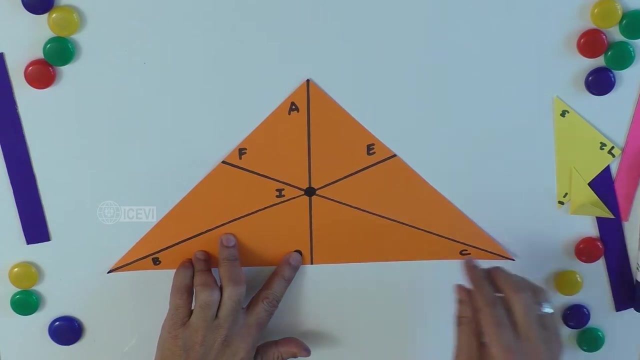 the angle B and the angle C and they are going through a point which is called as the In-Center. Now, unlike other centers like Circumcenter, Orthocenter, etc. In-Center has a special characteristic: Now you can form a full. 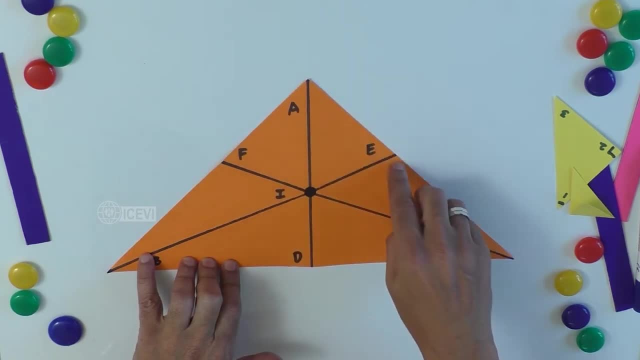 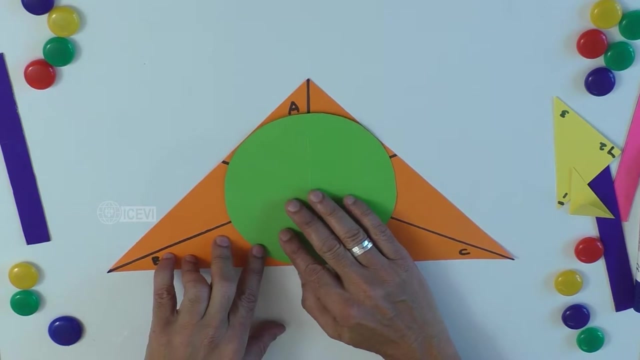 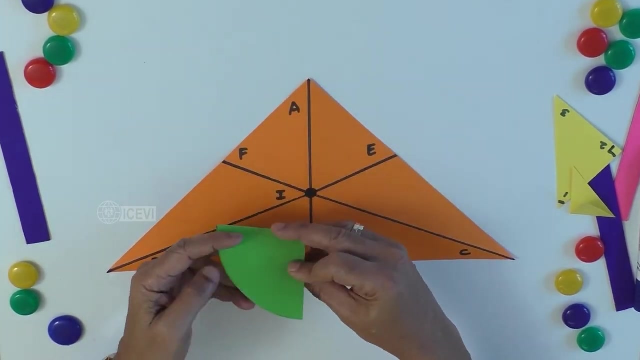 circle inside the triangle with In-Center as the center. Now we have to demonstrate this. So what we have done, for simplicity, we have made a circle inside the triangle. This is the full circle that you can get inside the triangle. Now take this circle, you fold it and make a semicircle, and then again. 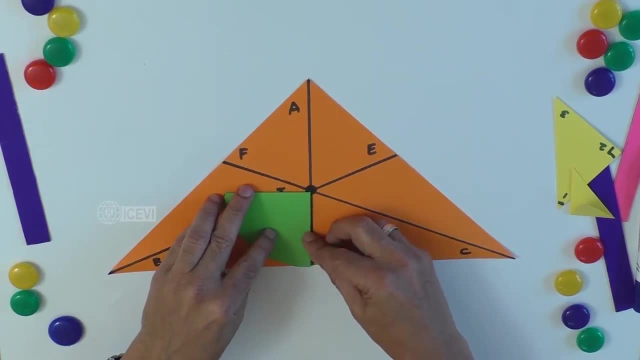 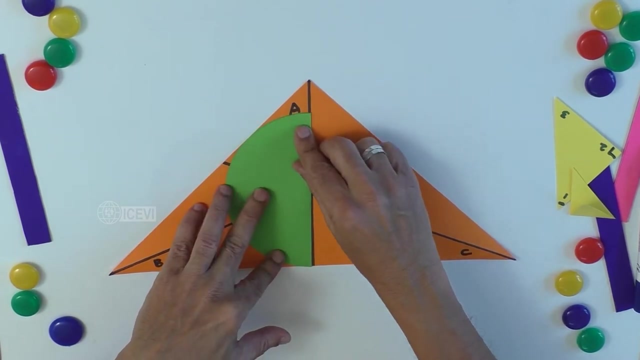 fold it. Now you can notice that the center of the circle and the In-Center of the triangle are the same. Now you can keep the diameter of the circle in such a way that it is coinciding with the line AD, one of the 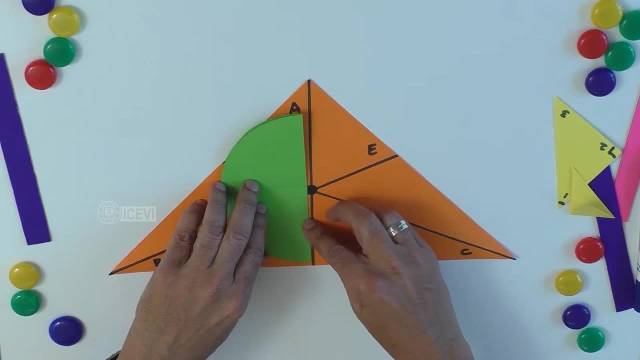 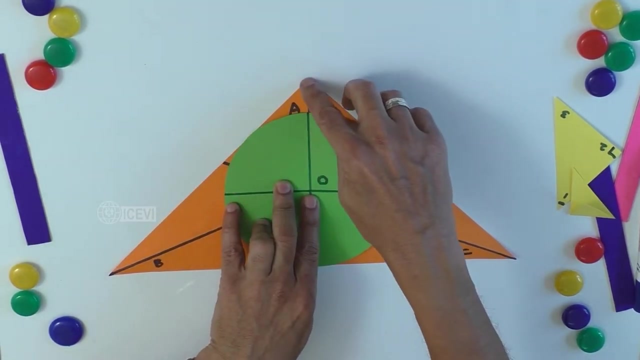 angle bisectors in such a way that one end of the diameter is at the point of the circle. Now you can note that at the D the circle is the base BC. Now, similarly, the circle will meet two points, one at the side a, B and another at the side AC. Now we may be tempted to 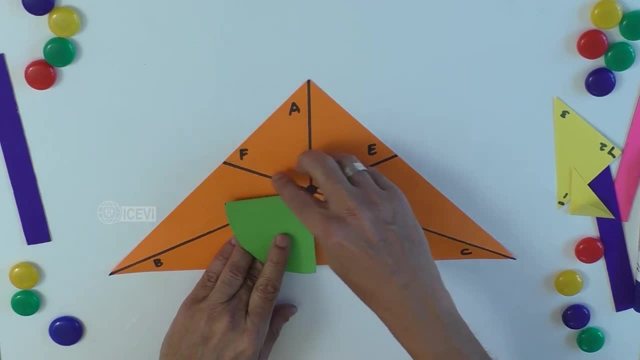 say it isn't happy to cooperate. now the circle feeds into two adjacent points to our center. that, IF IE become the radius of the circle, need not be. the circle is meeting at two points which are different from the points F and E. now how to find out? 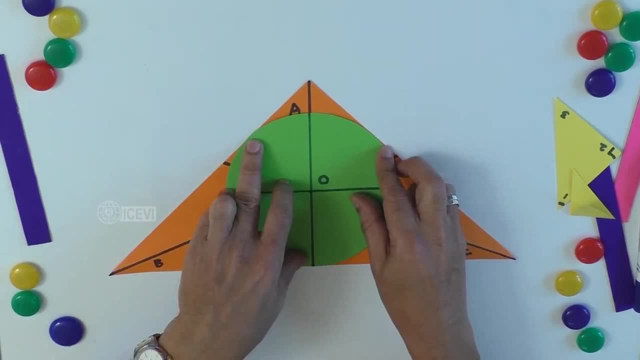 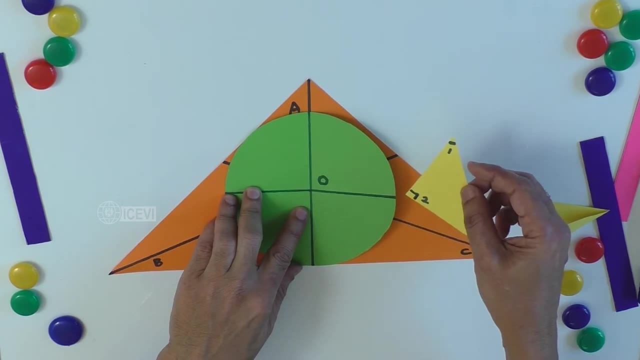 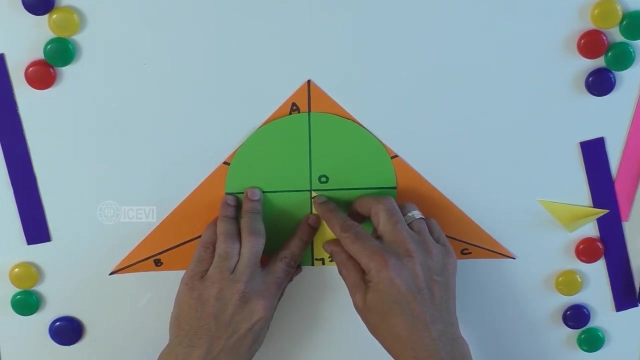 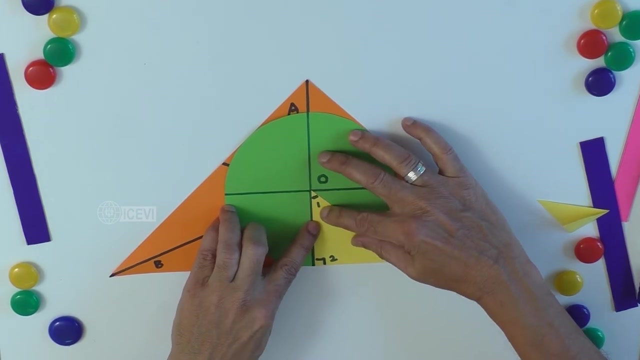 that point you know. you can find out the exact point through another special characteristic. this strip with right angle is formed in such a way that angle one, the vertex, is pointing at the center of the circle, which is the in center, and you can notice that the other end is seated on the side B, C and at the point. 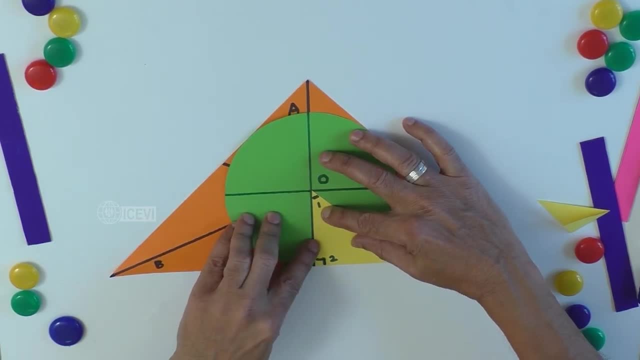 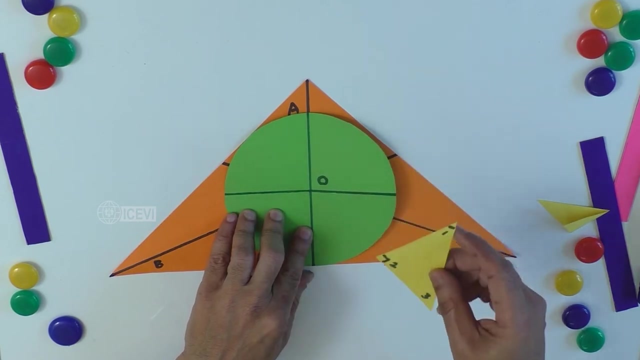 D, where the circle is touching the side BC. so what is the special characteristic here? at the point of contact, the circle is making 90 degrees. at the point of contact, the circle is making 90 degrees. let us try to find out in the case of other sites too. so angle one is pointed at the center. 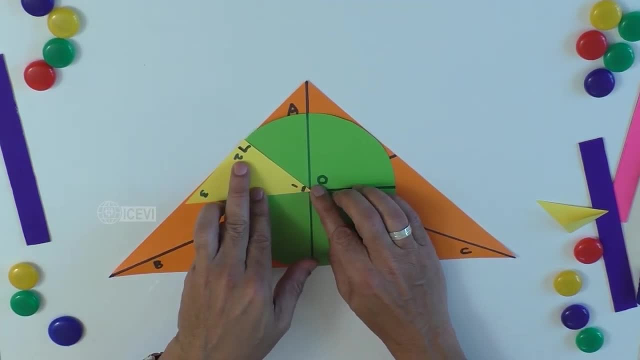 so you place the right angle in such a way that angle one is pointed to the center of the circle, in such a way that the right angle is formed at the side a, a b, so it is meeting a point at a- b. you can notice that that is different from the point f. 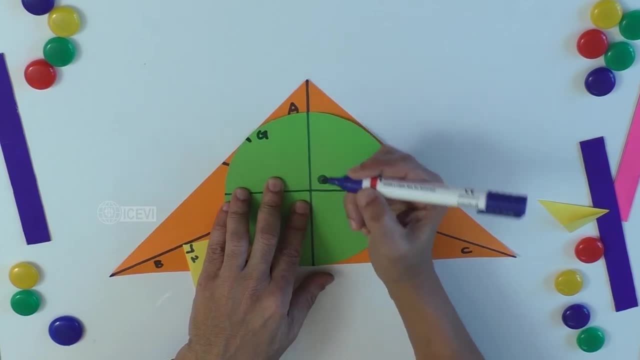 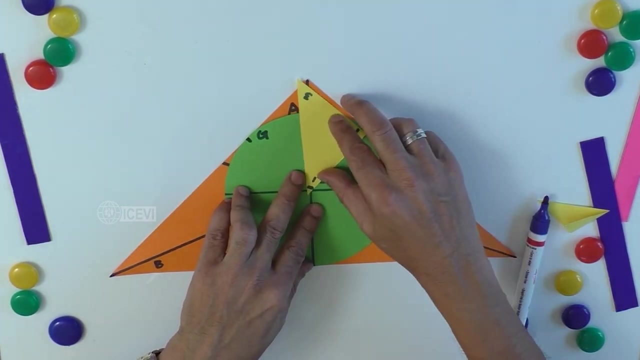 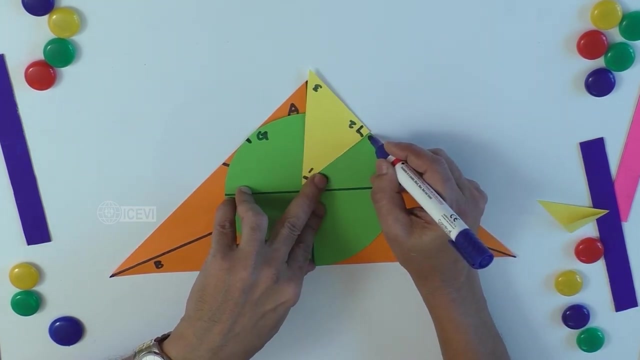 now, let us call this point as g. let us call this as g. similarly, you have to find out the other point of contact of the circle at the side ac. now, what we have to do, keep the angle one to coincide with the center o and you can notice that at the point of contact this, 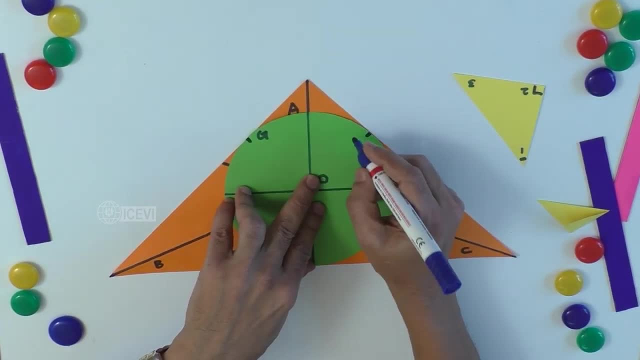 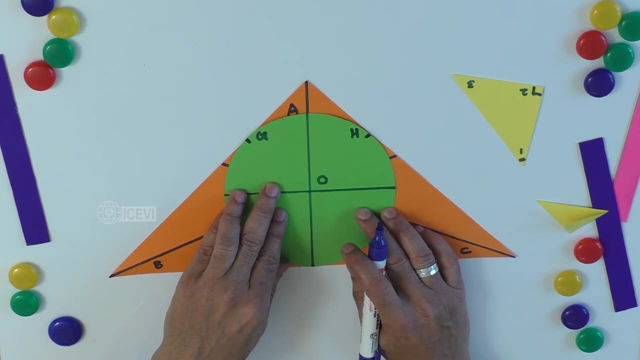 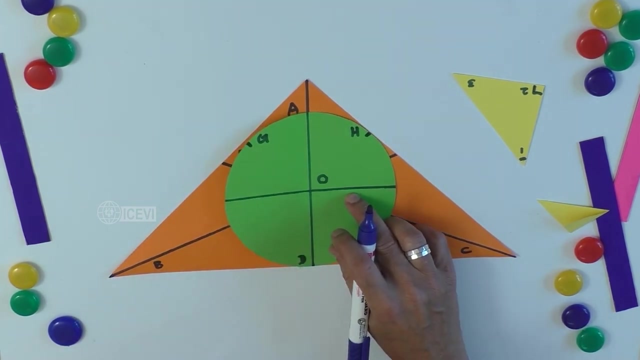 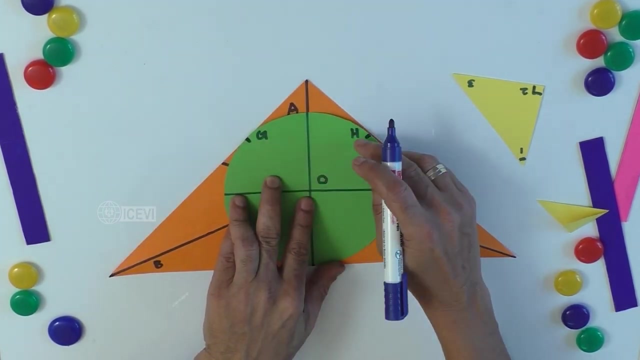 circle is making 90 degrees, so you call that as h. so the three points of contacts of the circle inside the triangle a, b, c. at the bottom, that is d, that is at the side b, c on the side a, b, it is at point g, now at the 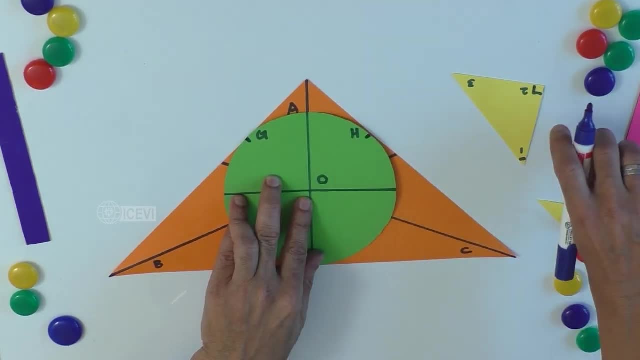 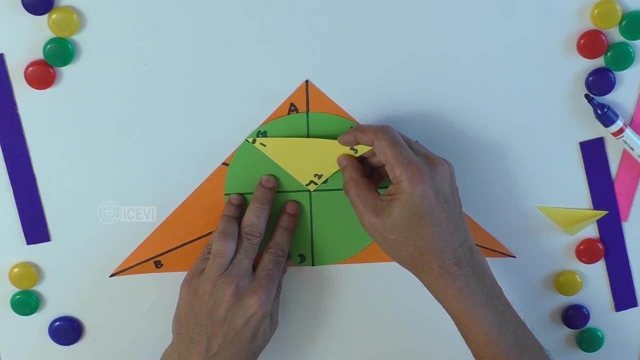 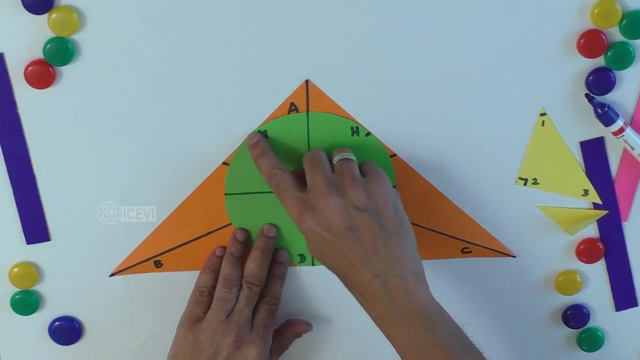 side a c, it is meeting at the point h. now you can notice that o h, which is equal to o g, which is equal to o d. so this is how we find out the in circle of a triangle: by forming the in center. so when you form the in center, 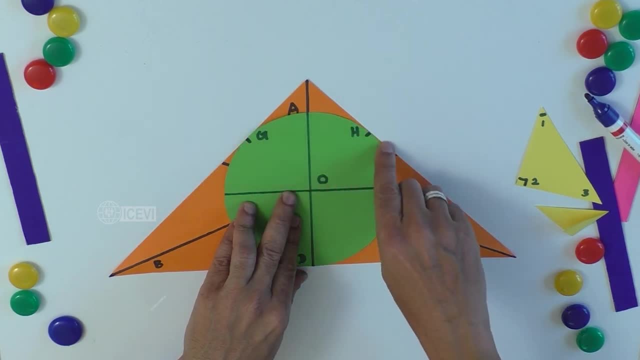 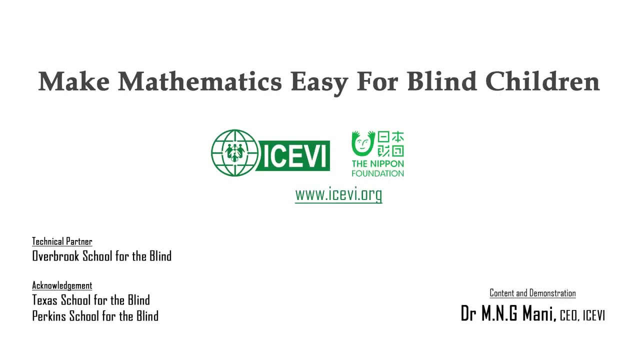 of a triangle, then this is the largest circle that you can get inside the triangle you.